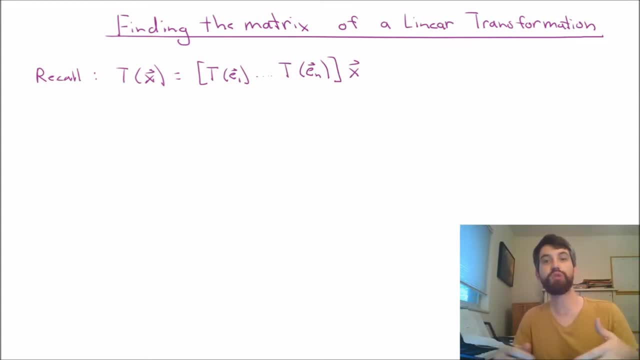 video was that this formula described for us the matrix of a transformation. In particular, if you had some transformation t and you knew what that did, then the matrix for it was going to be given by every column of the matrix is what the transformation does to one. 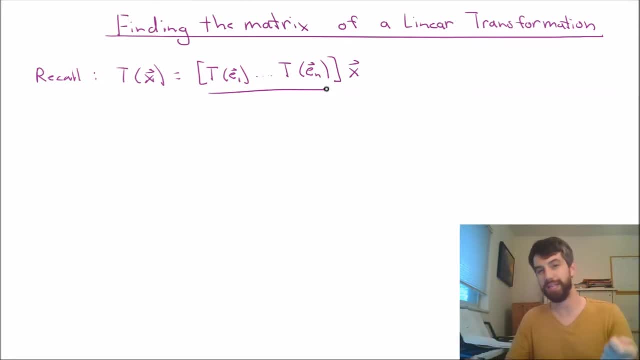 of the standard basis vectors, the e1 down to the en. Now, this is quite remarkable because, if you think about it, a transformation tells me what every single vector does. There's infinitely many vectors out there, that is" it tells me what every single one of them does. Yet what we've learned is that, if I know, only 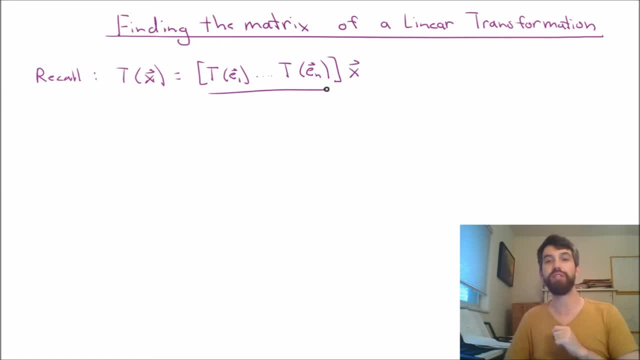 n pieces of information, namely what the transformation does to these n different vectors. if I know that, then it's sufficient that I can describe completely what my transformation is going to do, simply by knowing what it does to just n different vectors. So now, if I describe to 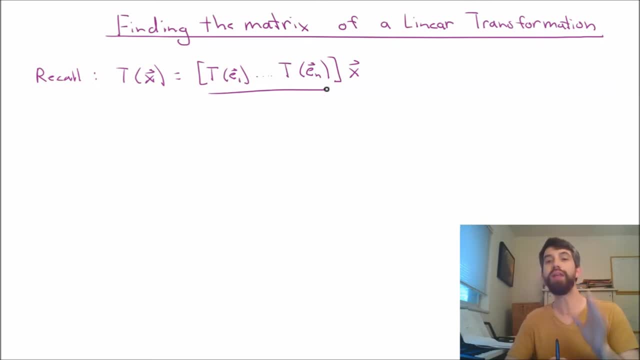 you some transformation. you should be able to figure out what its matrix is just by computing. what does the transformation do to the standard basis vectors? So, as an example, I want you to consider the idea of counterclockwise rotation. So that's my example. It's going to be rotate. 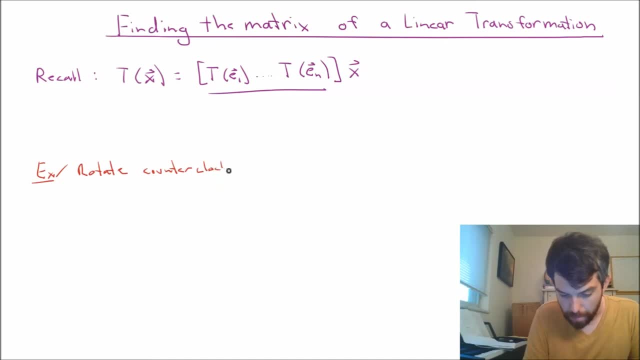 counterclockwise by some amount- theta- And we previously had sort of a visual description that made us think that this really was a linear transformation. but but now I want to see why it is a matrix transformation. So I'm going to give a little bit of a visual description for this. First I want to put my two standard. 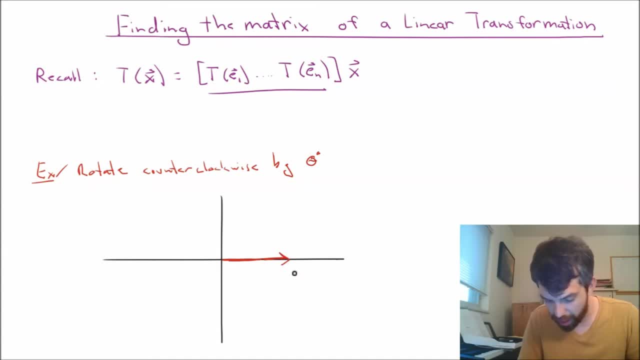 basis vectors on there. I'm going to draw them kind of long. There's my e1 that has the components 1, 0. And then up here I'm going to draw my e2.. That's going to be e2 and e2.. 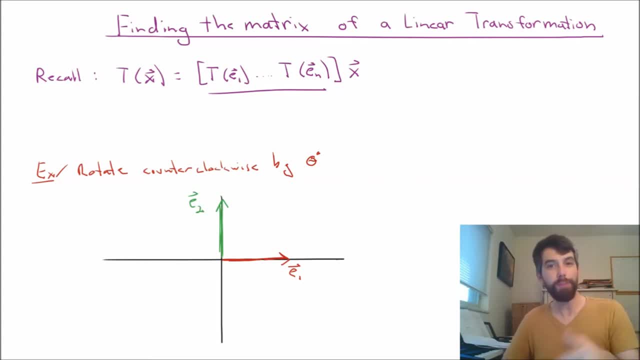 And then his components 0, 1.. Okay, so let me apply my rotation and see if I rotate counterclockwise by theta, What does it do to the e1?? Well, maybe my e1 goes to some amount like this where I've got an angle of theta inside of it. So this particular vector is: 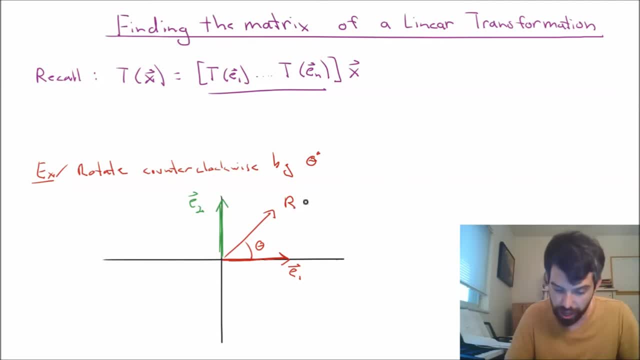 the transformation. I'll label the transformation r for rotation. It rotates it, and the vector e1 goes to this vector r of e1.. Well, we've seen this kind of triangle before. Indeed, you can sort of imagine, if I sort of overlay the, the circle here, if I do this projection, the x component, this portion here, 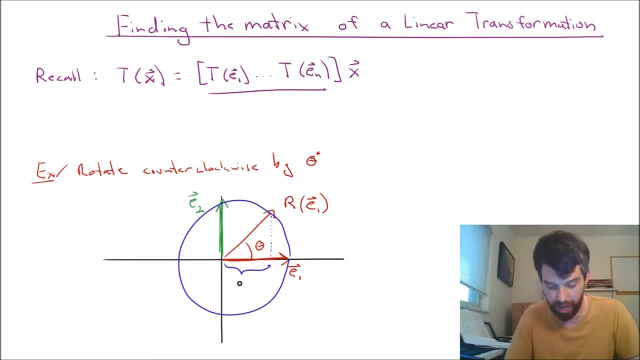 that is well. how does my trigonometry work? That's my cosine of theta And then the height of this point. this is going to be sine of theta. So if I want to out what my R of theta is going to be, This is a vector whose x component is: 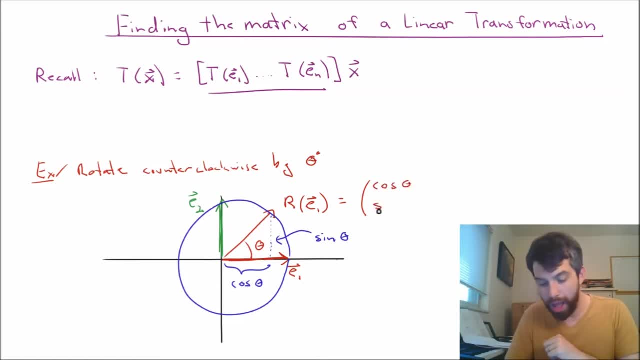 cosine of theta and whose y component is sine of theta. So in other words, we were starting with this one basis vector, the e1, and then we were rotating it up some angle theta and we were saying: what does the transformation do? What is the final coordinates? In other words, we were asking: what is the T of e1 and we 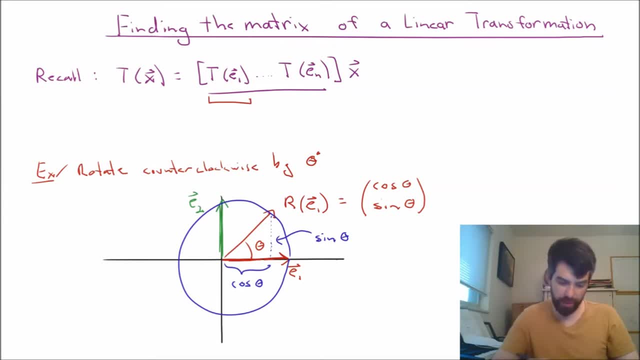 have gotten that it's cosine theta sine theta. I could quickly repeat much of the same story here. for the other one, My picture looks a little bit distorted, but this is going to be the rotation of the vector e2. and then, if I want to figure, 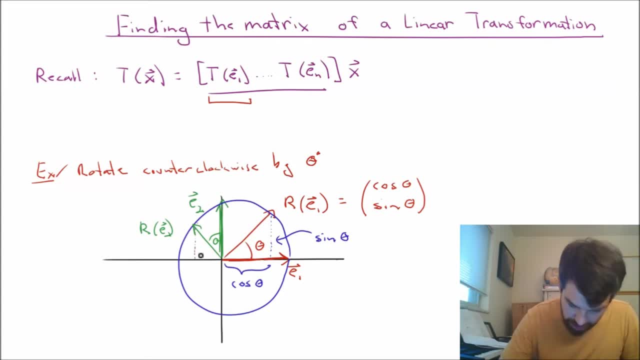 out what the x and y coordinates of that. that's doing this bit of trigonometry. here The horizontal is going to be sine theta, but it's in the negative direction, so it's going to be a minus sine theta. And this height here is still positive and it's going to be represented by 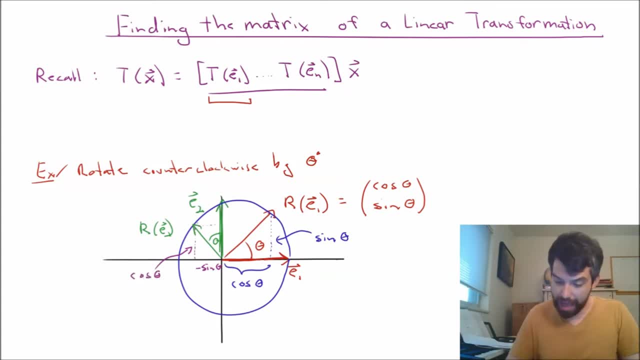 cosine of theta. So, in other words, what I have with the R of e2, its description is going to be: its x component is minus sine of theta and its y component is going to be cosine of theta. and there we have it. So now, if I really want to, 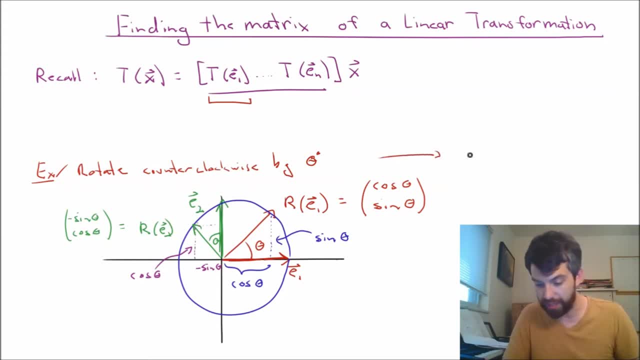 finish off what my proof is going to be. it's going to be this: that the rotation of any vector x is going to be given by some matrix, and the matrix is the one whose first column is the rotation of the e1. so that's going to be. 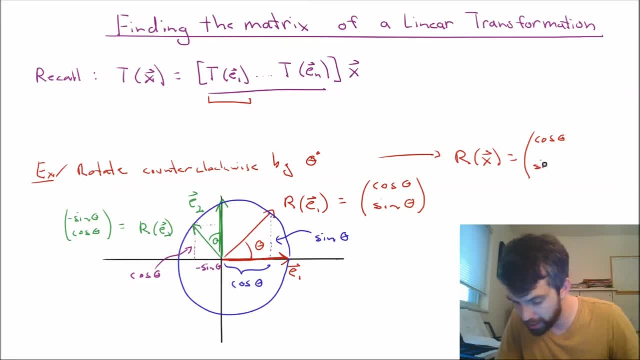 cosine, theta sine theta, and whose second component is going to be the rotation of e2, which is going to be minus sine theta, cosine of theta, And then it's that entire matrix that we have multiplied by the vector x. So this here is our 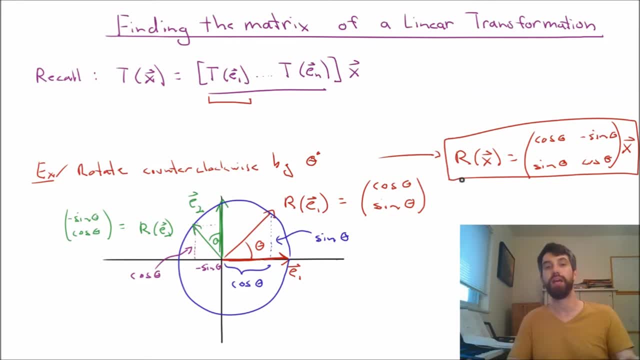 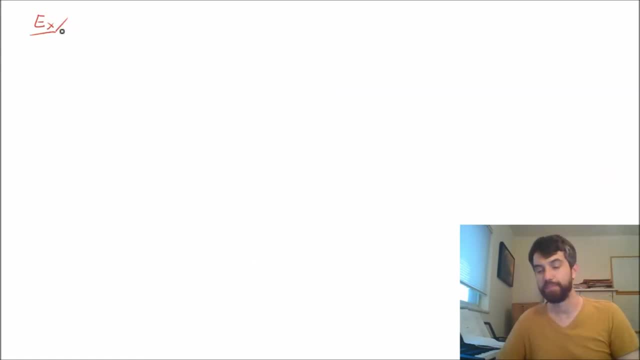 rotation matrix, or at least our rotation matrix for rotating counterclockwise. Alright, let's see one more example of this. I'm just gonna make something up. How about this? This is a transformation from R2 to R2, and what does the 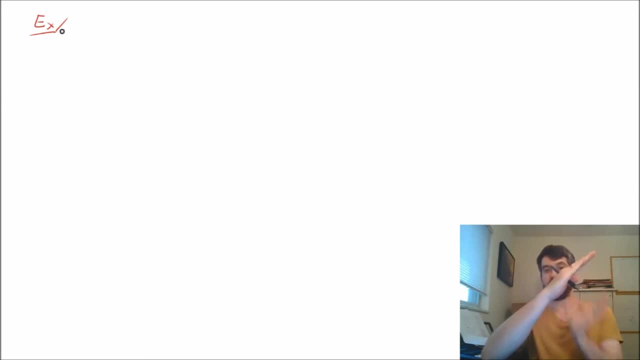 transformation do? First of all, how about it flips over the line y equals x. So any vector sort of flips over the line y equals x. Then how about? it rotates clockwise by 90 degrees. I just made one up. Let's try to figure out the matrix. 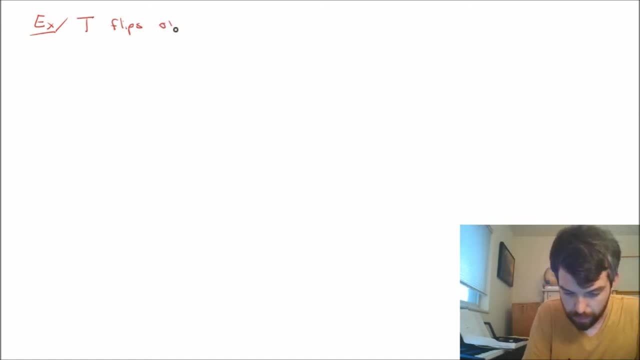 for that transformation. So to find the matrix for this transformation, we need to know what happened to the two different standard basis vectors. I'm going to do this one first. This is my E1, and its first step is to flip over the line. y equals x, I sort of 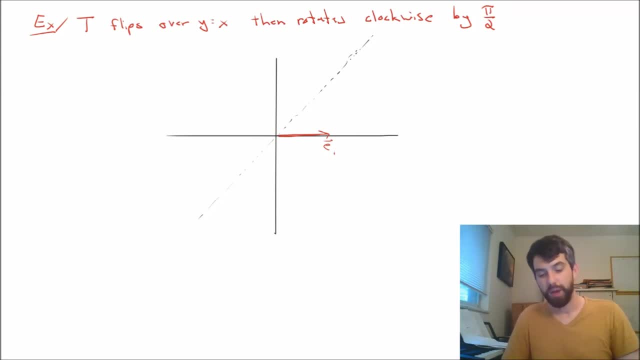 dotted that line in on my picture. Well, if I think about it, okay, we've got a line here and then if it flips over that dotted line, that's gonna be straight up. So that's gonna flip up to here. This is sort of like a preliminary stage. I'm not 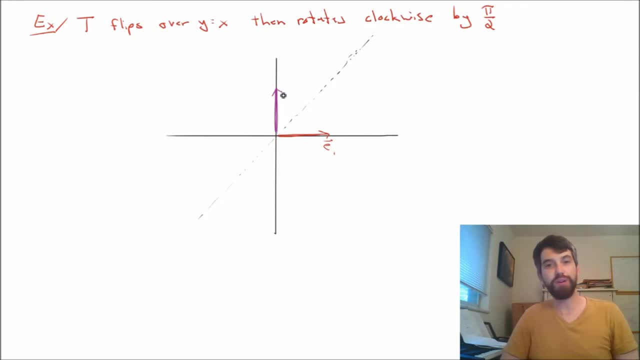 gonna give it any name And then after it's up there, it has to rotate by 90 degrees. So it's gonna rotate right back down onto the E1 if I'm rotating by 90 degrees, So this is gonna come right back down here and lie. 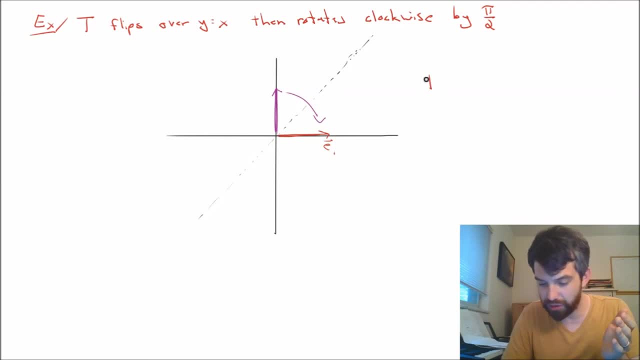 exactly where it was. So, in other words, my transformation is going to take the vector E1, and the combination of flipping it over y equals x and rotating it by pi over 2 takes it right back to where it started. So t of E1 is just E1. 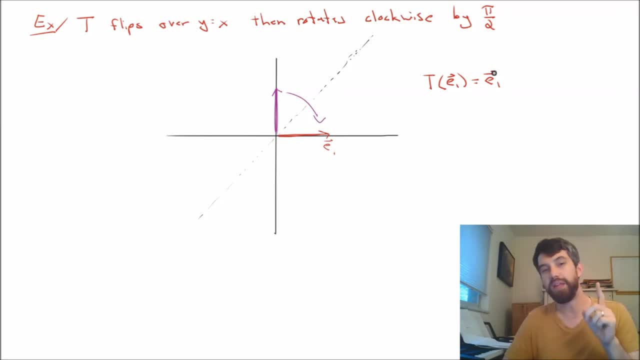 The transformation doesn't do anything to the E1. But maybe it does. Maybe it does something to the E2.. Okay, so now let's investigate what happens to the E2.. So I'm gonna put my E2 on. That's this. It's sticking straight up. There's my E2.. 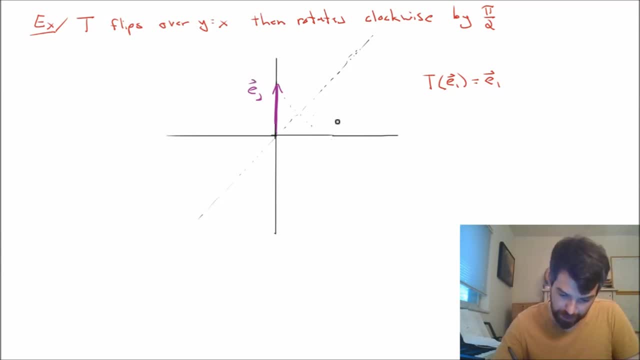 So then it's going to flip and the flip flips it down here and now I'll don't- I'm not gonna give a name to it, but it's that intermediate one sitting there And then it's gonna do the rotation by 90 degrees clockwise and that's gonna stick.